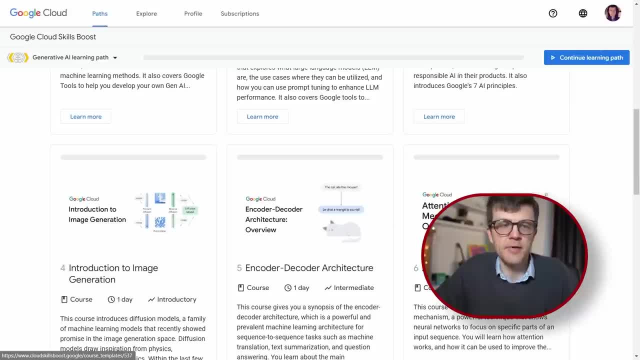 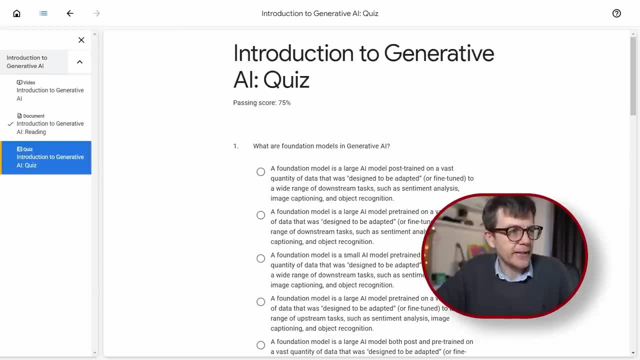 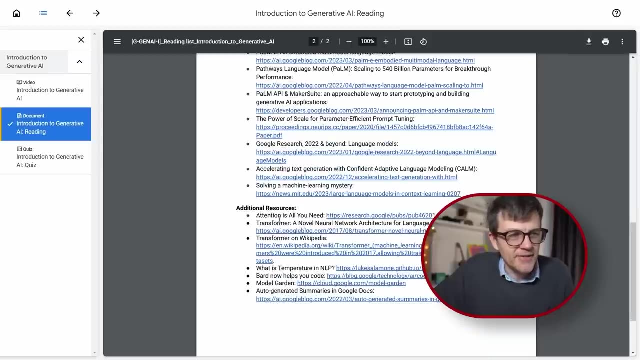 an overview of encoder and decoder architecture and an overview of attention mechanism. So this is a really important module, this one. Let's have a quick look. So one of the things I like about the first module is the reading list. It's quite comprehensive and it's good to see that it's got this. attention is all you need. 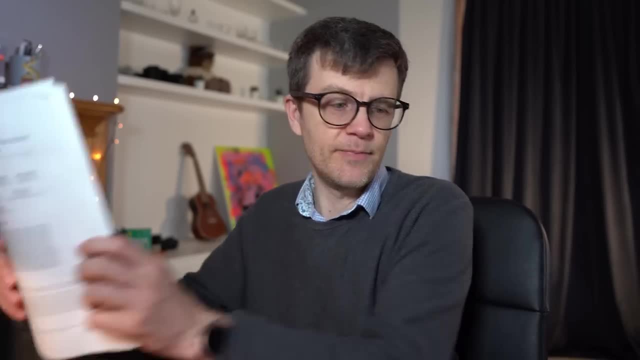 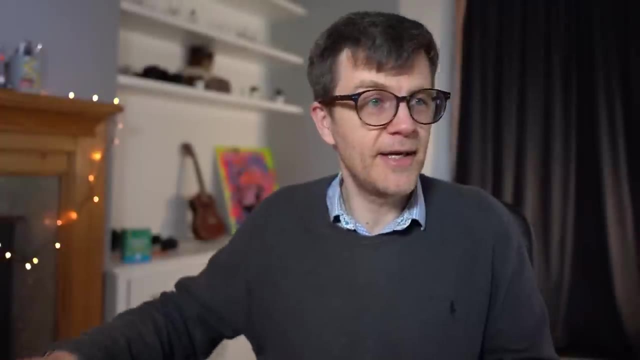 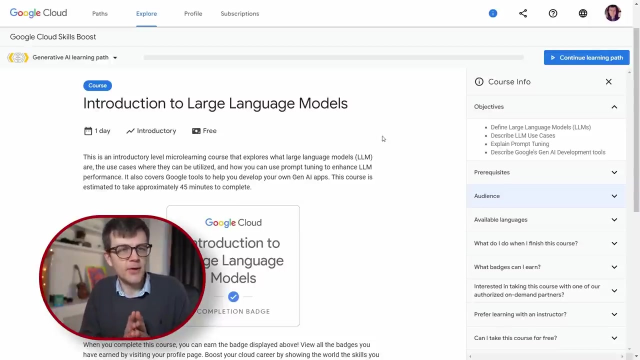 reference there. So that's this paper that came out in 2017, which really was responsible for a lot of the advances that we've seen in AI recently. So do the module, then read the paper. There's also a little quiz at the end too. Now module two. I really like module two because well, it's for. 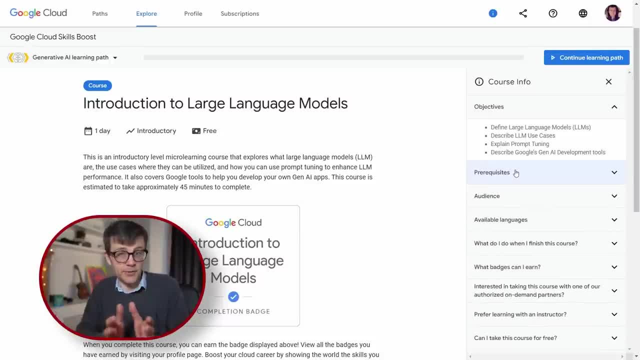 general education. It's for general education, It's for general education, It's for general audience and there's no prerequisite knowledge required. So it's a good overview of how LLMs work, which is really important, because I'm no expert on LLMs, but I think there's quite a lot of confusion. 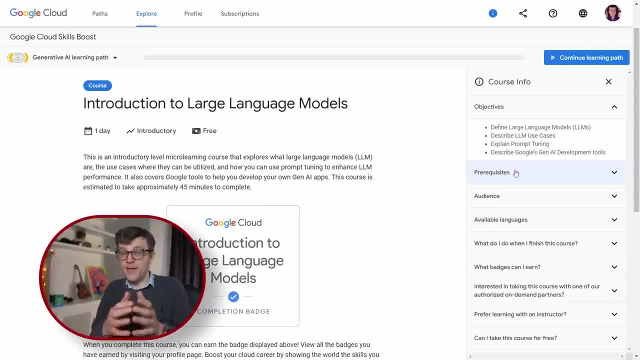 about. you know how they work, what they're capable of and especially what they're not capable of, and you can see that a lot in sort of popular newspapers and magazines and articles that have been written in those publications and on websites where the journalist hasn't really 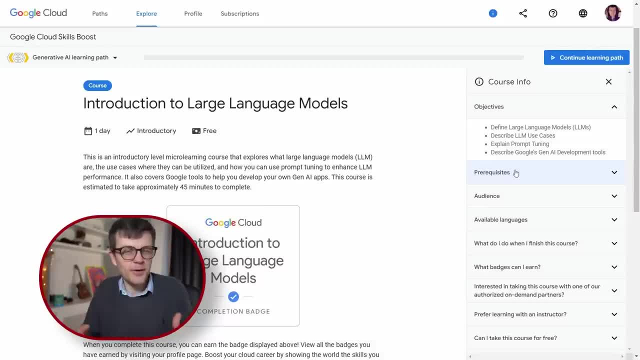 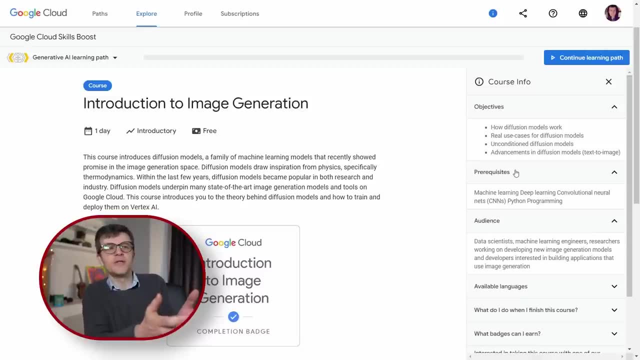 understood how they work or what they do, which leads to sort of a lot of confusion amongst the audience as well. So that's a really good module and it's for a general audience, which is interesting, because then when we get to this module- which I also like- the introduction to image. 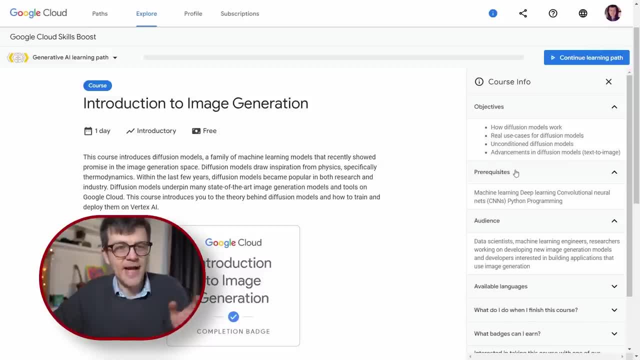 generation. this is, for it seems, a different audience. So this has prerequisites of machine learning, deep learning and CNNs and Python programming, and the audience is for data science, data scientists, machine learning engineers and researchers. But don't let that put you off. If you don't fall into that category, then you know, image generation is really interesting and 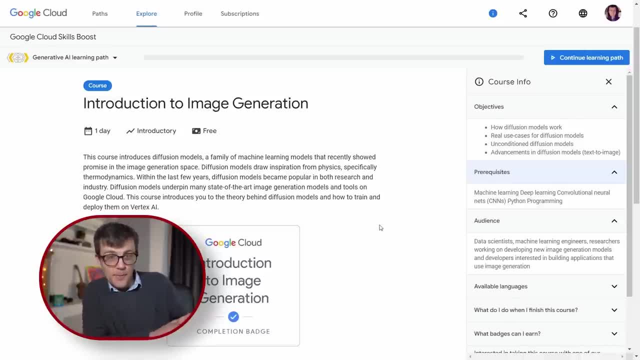 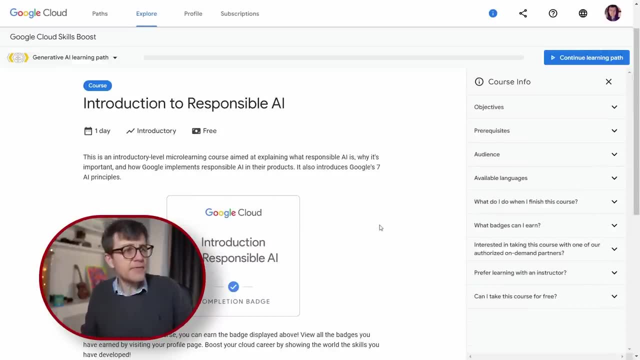 diffusion models are really interesting. So I think that's a really good module. So you know, I think if you've moved along the path and you've reached this point and you want to know how they work, take a look. I don't think you'll be disappointed. And then, finally, the other. 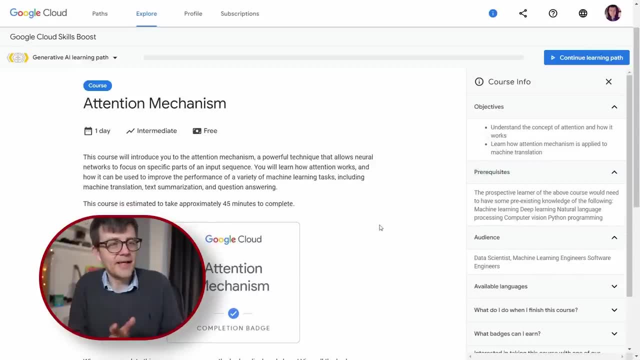 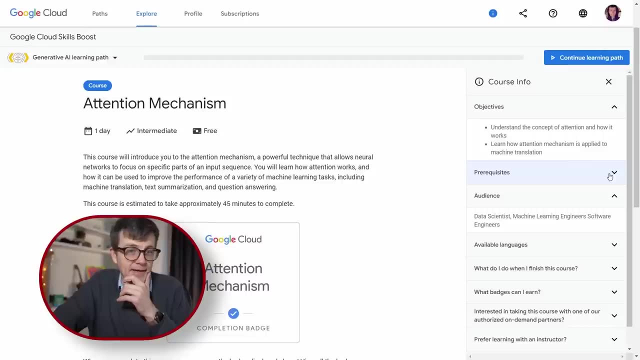 one I wanted to have a look at was the attention mechanism, which is such an important topic on generative AI that it would be silly to miss it out, even if you don't really fall into again the audience that it's aimed at, which is data scientists, machine learning engineers and